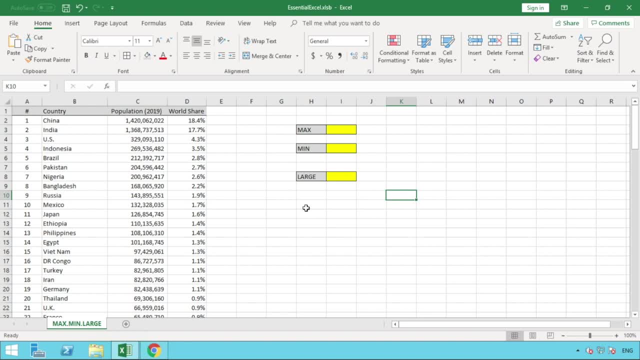 just be of interest to you, but it's as the data set came. it shows you what that population is So well. WorldShare shows you what proportion of the global population that country takes up. So maybe to explain that a bit simpler, so China, in row number 2, is the largest country. 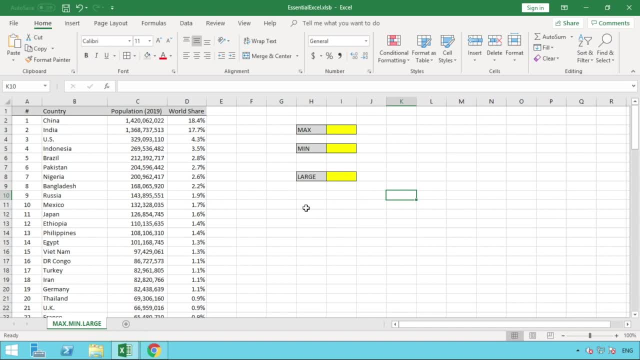 by population, with a population of 1.4 million people, and this 1.4 million people is 18.4% of the global population. So that's what that means. So it might be of interest to you to see that. it's quite interesting facts to see. but for the purpose of this demonstration, 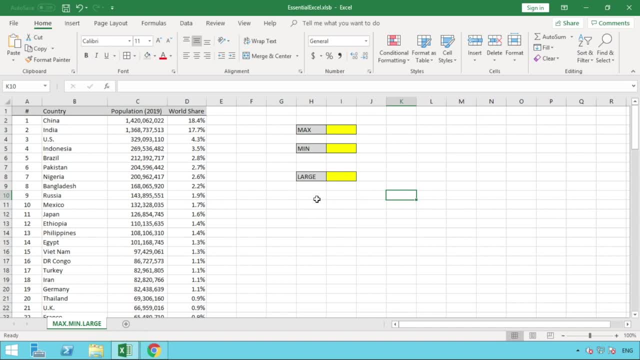 we'll just be using column C, So let's look at some of these functions in column H, or that's where they show the name. We'll work on max and min first and then we'll go into large, as that's a bit more detailed. 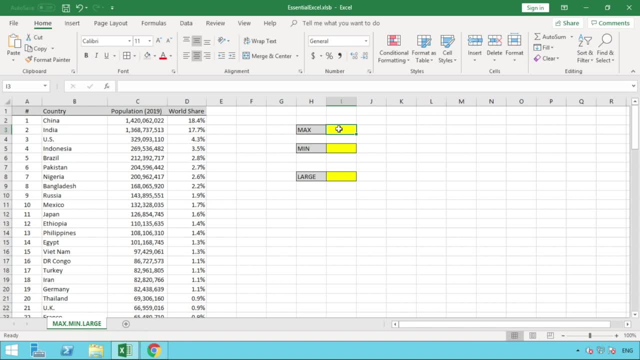 and a bit more to look at in that one. So the benefit of max. so, as it indicates, max is going to show us the max or the largest value in a range of data. So, quite simply, if all we do to do that is we enter our equal sign and type max, open our brackets and then 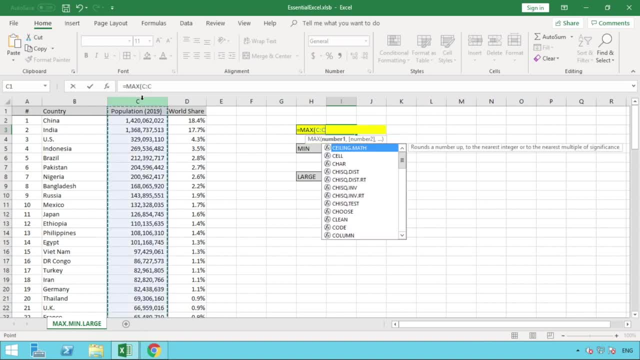 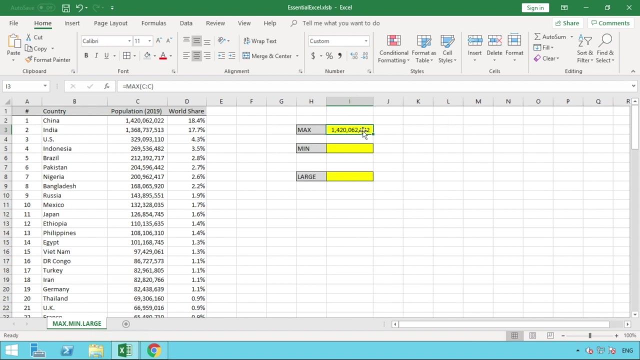 we can select column C. Here we go. Now let's look at column A. We're going to look at column A for this example because we're looking to find out what the largest population size is, And then when we hit enter, Ok, it gets there eventually And we might have to expand these cells slightly There. 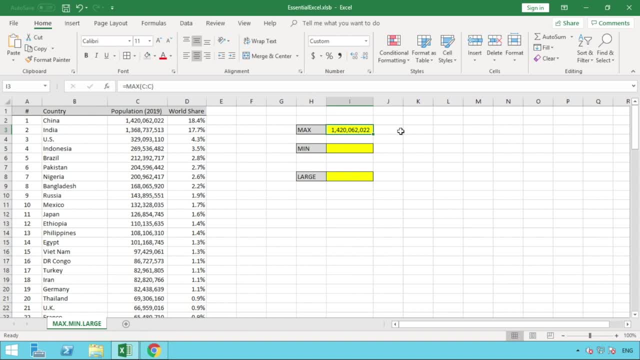 you go. So, as you can see, what it's done is pull through the max or the largest population size in column C, which is 15.5.. So that's what it's going to show us in column C. So, actually, 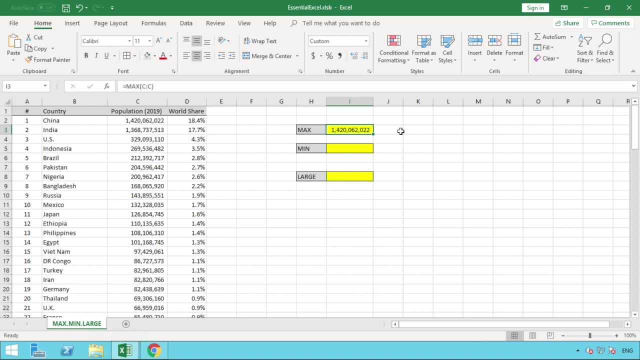 that 1.4 million for China, and so it doesn't give you much more detail than that. but at least what it does is it shows you what that largest population size is. I guess for our example here, our countries are all already organized in terms of the population size, so we can see the maximum straight there at the 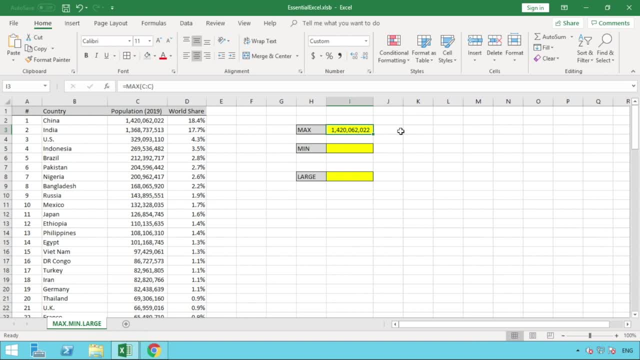 top, and we will be able to quickly find the other one as we move on to min, but we'll just show how min works as well. min does work in exactly the same way, and in order to do this, you enter your equal sign, min, and then open brackets. 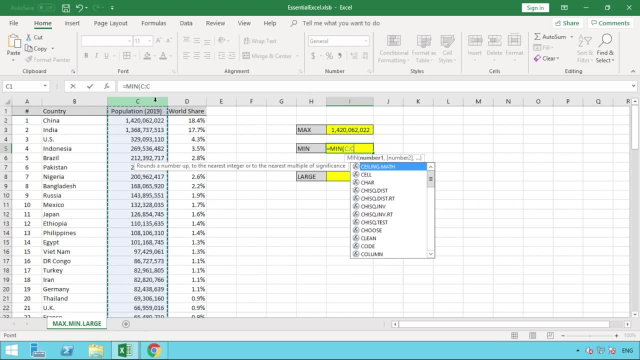 and then we can select column C and then close brackets, and it just takes a little while for it to calculate, as it seems to have done with max. but we'll give it a couple of seconds, cool, there you go. so the two form or functions work in a way that they work in a way that they work in a way that they work. 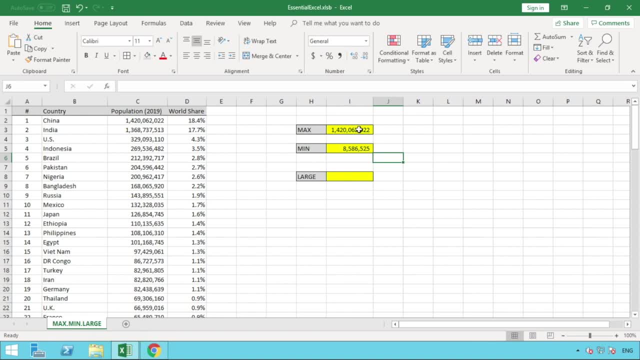 in a way that gives you, allows you to quickly summarize and compare these two numbers, so we're able to find the max value, what is the 1.4 million, and the min value, that is, the 8 million, 8.5 million. well, actually sorry, no, but I've. 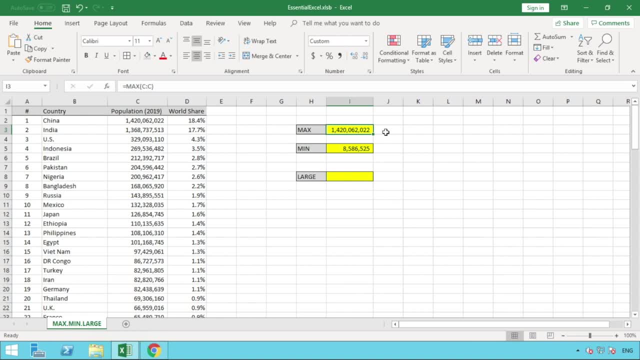 been saying 1.4 million for max. that is completely wrong. that's not 1.4 million, that's 1.4 billion. so yeah, that's, the population of China is 1.4 billion. sorry, that's a quick correction there. yeah, so then that makes more sense here when we 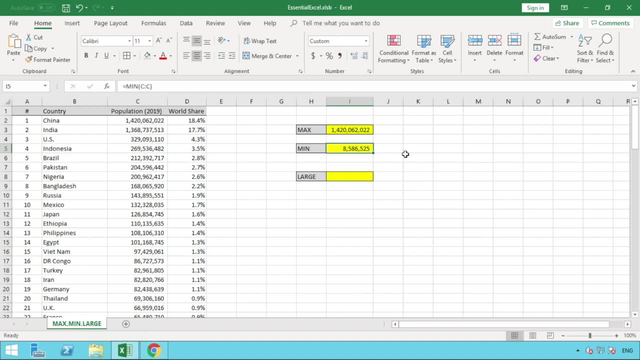 can see the 8 million for as our largest population size in our list and if we scroll to the bottom of our list to number 100, there we go, we can see that value: of 8.5 million. what's actually lines to Papua New Guinea as country? 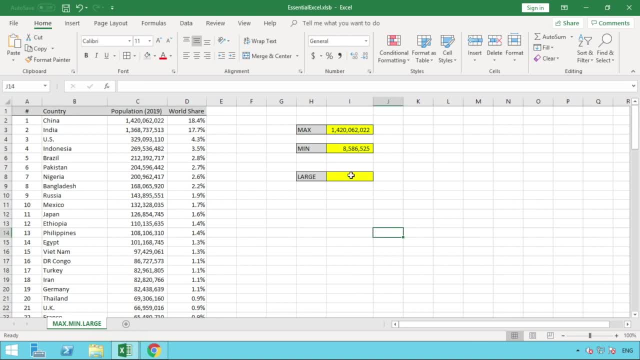 number 100- cool, so those two formulas are again really useful. allows you to do any quick summaries, such as we've done here if you need to, as a reference point, if you want to do any comparisons or even just to find what those largest values, where there's a quick way of. 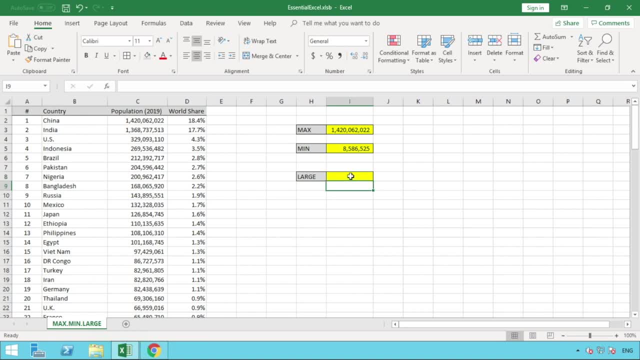 finding them. so we'll move on to large and large does? it? is a similar, similar function, although it has one more entry point, rather than just selecting your range. so we'll, we'll work. we'll go through and describe how it works as we type it out. so, as always, we enter our equal sign first and then we type our. 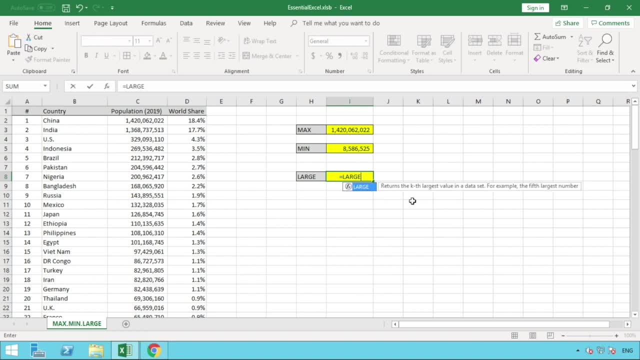 formula what is going to be large and then open brackets. so, as you can see from our little instruction pop-up that comes here, we have two parts to this formula: the array and then comma K. so, simply put, the array is the range of data we want to look at, and then K is. 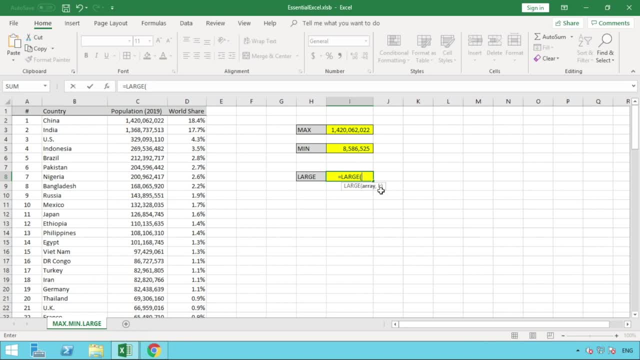 where we indicate what value we want to find. so to explain large, well, actually, let's put a formula in first. so what we want to do is use large to find the largest value in our range in column C. so in order to do that, we select column. 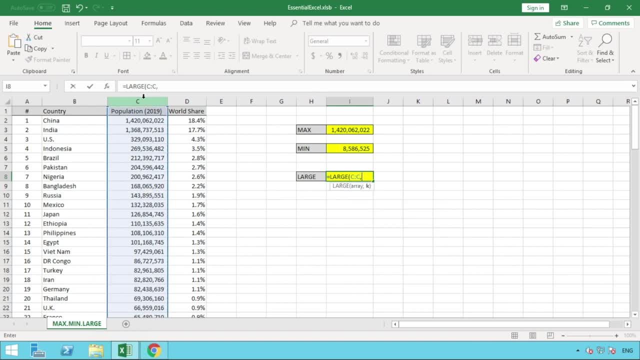 C, do a column comma, sorry, and to find the largest value we simply enter the number one and then what that number one indicates is we want to find the first largest or the largest, and when we hit enter to that, what we will find is that will then match the value we have. 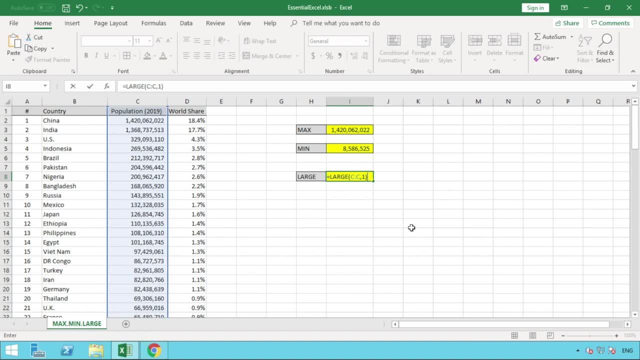 you for our max formula. what you see there in row 3 or column I, what is our 1.4 billion population? that we now know it sits and belongs with China and we can see that by referencing our table on the left hand side. so once this formula is, 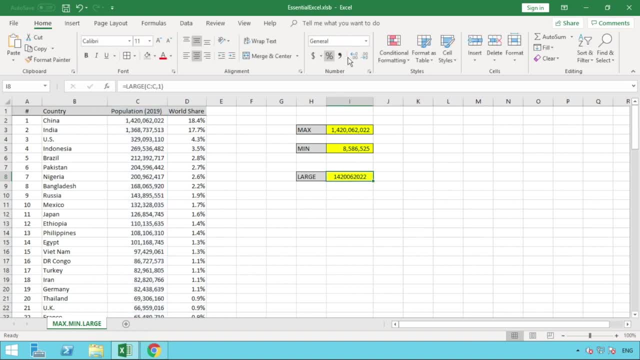 taken. perfect, and let's just just do a tiny bit of formatting just so that looks this easy to reference. perfect, so you can see now that large is exactly the same as max and by entering the value of one. that is exactly what you'll do. you will. 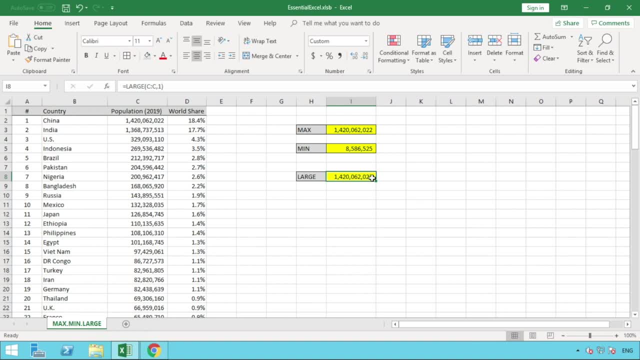 just find the largest value in that range. so why use large? well, the benefit we have of large as it enables, enables us to go a bit more, get a bit more detail. so, rather than finding the largest value, we're able to find the second largest value, and in order to do that, we change the value or the number. 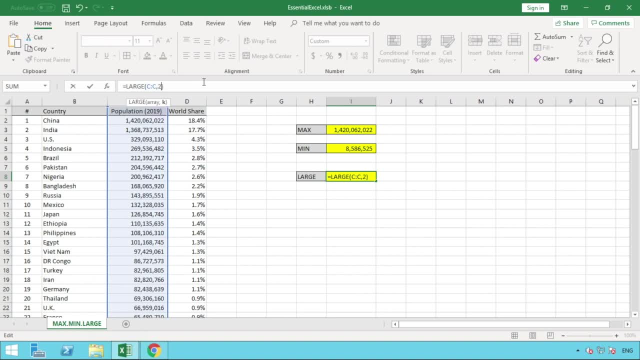 of one to the number of two, you, and hit enter on our formula and then what you'll see happens is what it will this time do is what it will: rather than just returning the largest value, it will find the second largest value and which, in our data set, we can see is going to. 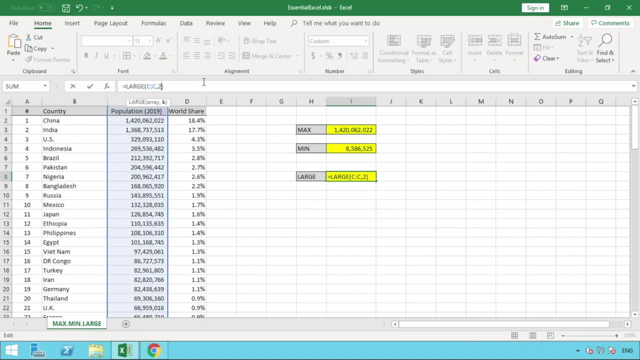 be the population for India, which is 1.3 billion or just short of 1.4 billion. even so, once we get out of this formula, there you go. we can now see we've got the 1.3 billion there and large works there with the same, and, and if you want to find the third, 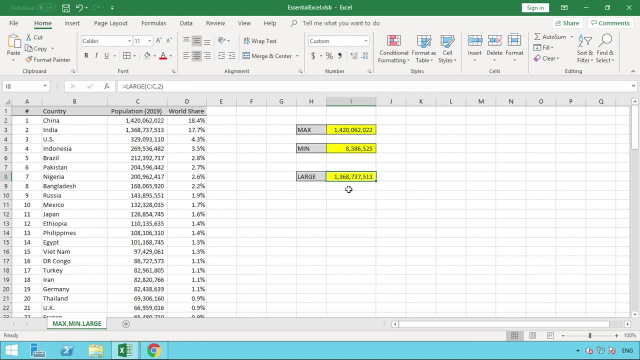 largest or the fourth or fifth, you simply all you need to do is just update that and that second piece of information, the number. so in our example of the example, you then change the two. what we need to do is change that to the desired number that you wish to find. 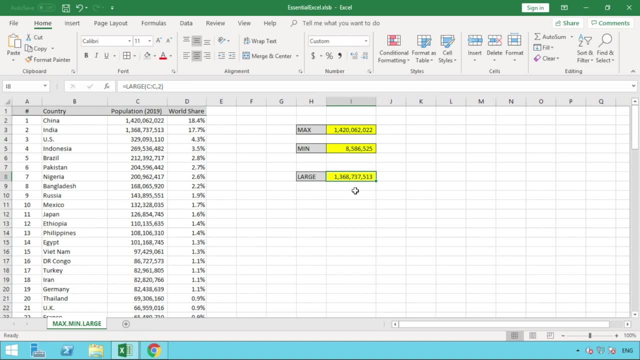 large is really good. if you wanted to do a quick table summary to demonstrate, then the top 5, or the first, second and the third largest, or if it is in terms of time, like you could say, the fastest times, and that would work really well as well. so there you go. there's the three formulas that we want to look at today. we hope that was. 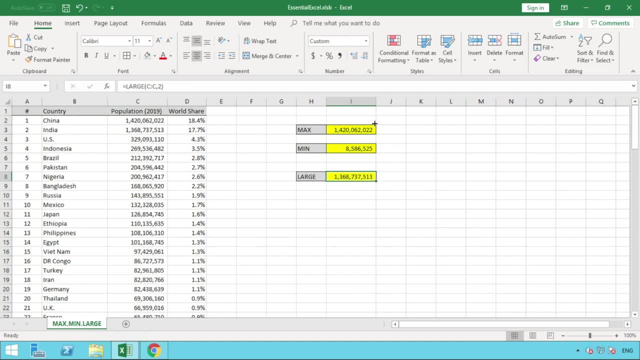 really useful for you, as you, as we sort of touched on earlier, these numbers. on their own again, they can be very useful and allow you to summarize. but another step we could take is to is to now say, okay, we found the largest value or the second largest value. how can we return? what country? 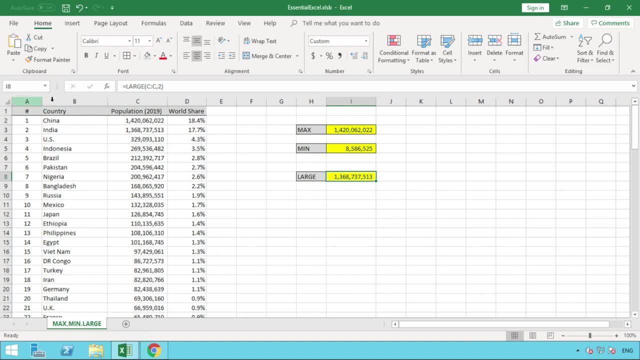 that belongs to. so, as you know, because what the data here we can quickly reference and say, okay, well, 1.368 billion is India. but had you not got this data to the left here, or it was a larger data set or those values went at the top- you would then need to manually search through the data to 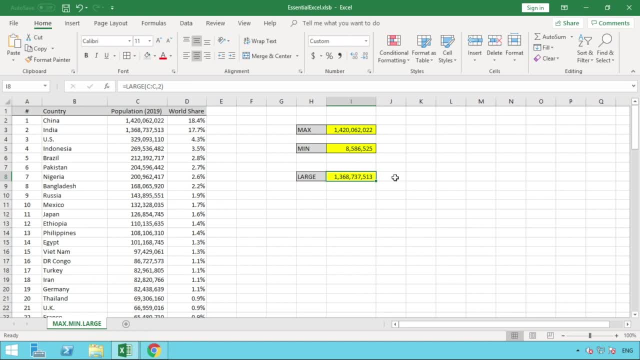 find that country. but we do have a step that we can use to use this information and return the country it aligns to, and if you'd like to look at that or if you'd like us to cover that topic, you can do that by clicking the link in the description below. and if you'd like us to cover, 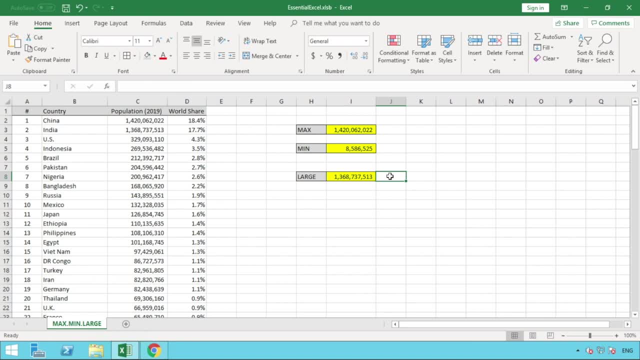 that topic. you can do that by clicking the link in the description below and if you'd like us to cover, please give this video a big like. also comment below to let us know that you do want to see that video and if you haven't already, please remember, subscribe to our channel. we have lots. 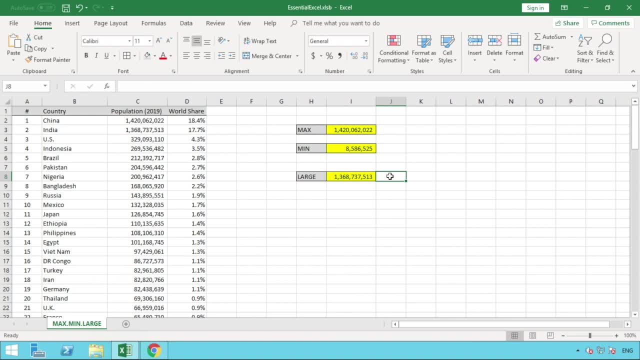 of videos that are coming up, and we're going to start diving into some more technical stuff and bring all together. bring together all the stuff we looked at so far, so make sure you don't miss those. and lastly, we also do have a facebook channel, and so links to that are in our description. 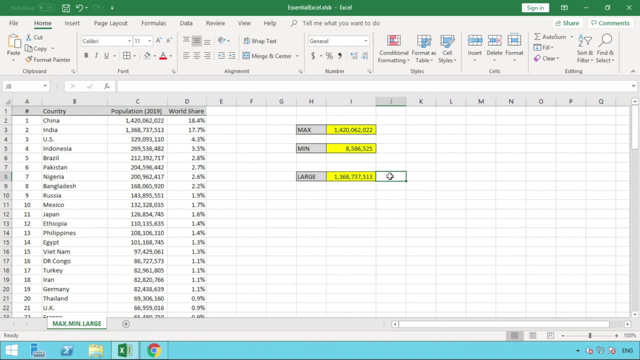 in our facebook channel we do, or facebook page we do- also have a members group, so you can currently join that group for free, in which you can talk and discuss ideas with other people who are trying to answer and ask questions in excel, and obviously that's where we'll post a lot of our topics as